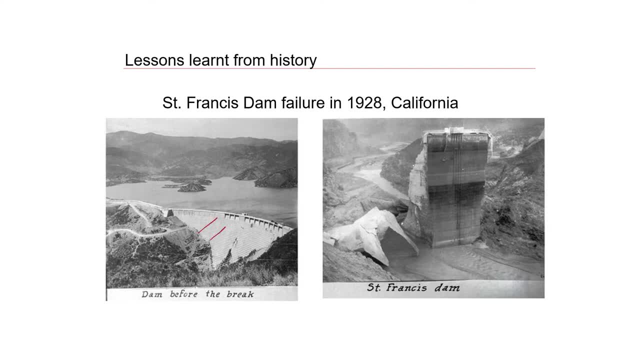 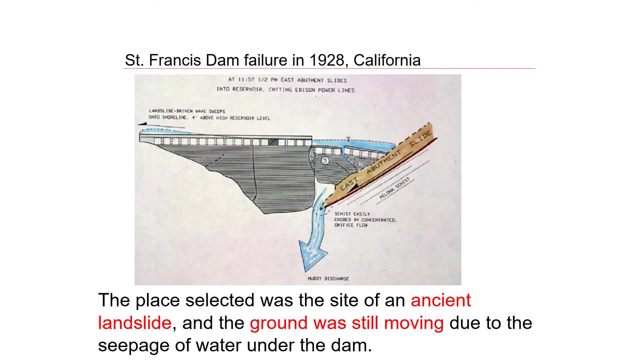 important. This is the dam that was designed and built to hold water. Three weeks after the dam was completed, there was a huge failure, So the dam collapsed. and this is the picture of a dam after it was collapsed. So what happened After the failure? they did very thorough site investigation to find out the reason. 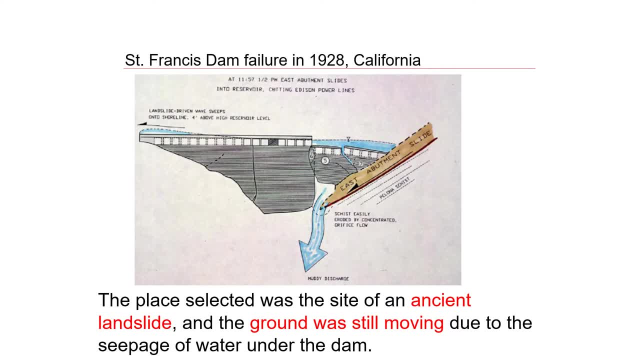 and apparently this dam, or part of this dam, was built on ancient landslide. So in fact that part of the slope was unstable because many, many years ago it failed as landslide, but because the previous site investigation didn't pick it up. so the dam was built on this potentially unstable slope and when 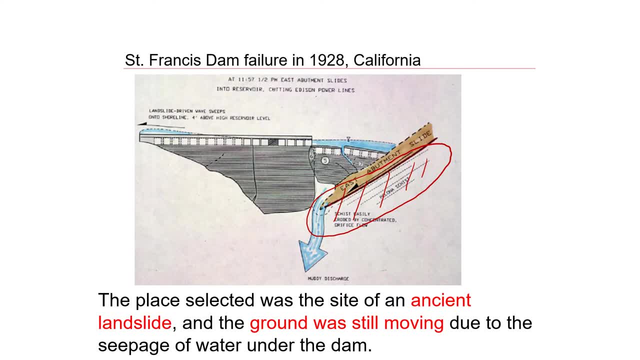 the dam was filled with water. there was some seepage through this part of the dam because this soil wasn't as hard as the soil here on the left hand side. So this part was ancient landslide that had undergone some movements over time and it made the soil very, very soft and loose. 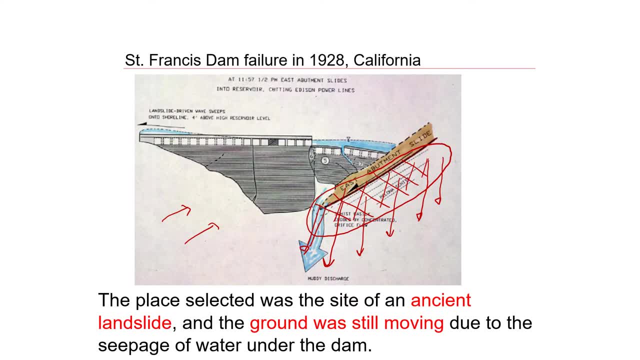 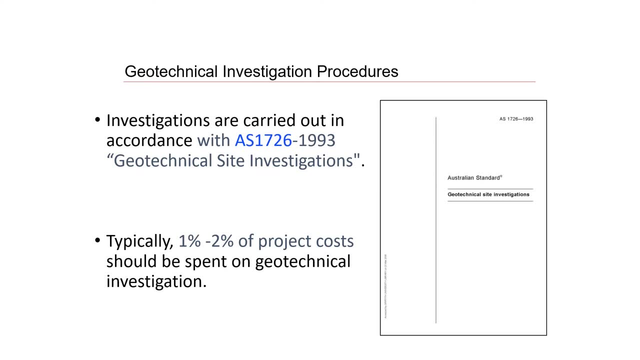 So this is the major reason for this failure To do site investigation. we need to follow a standard and in Australia it is standard as 1726.. It's a very important document that describes what type of site investigation needs to be conducted, Typically for large projects. we spend about one or two percent of the project cost on site and site investigation. 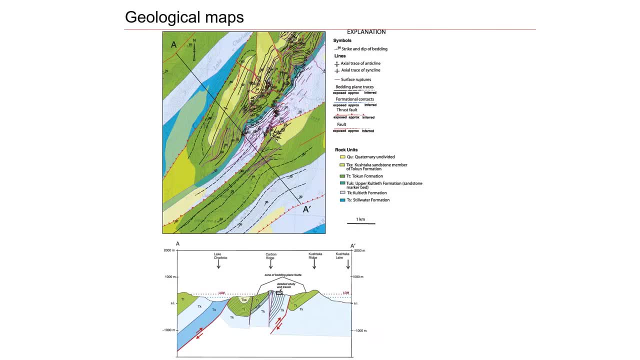 So the first thing that we would like to do before we start our site investigation is to find geological maps of the area that we would like to investigate, and this slide shows the example of a geological map. You can see that this map has different colors. It has blue color. 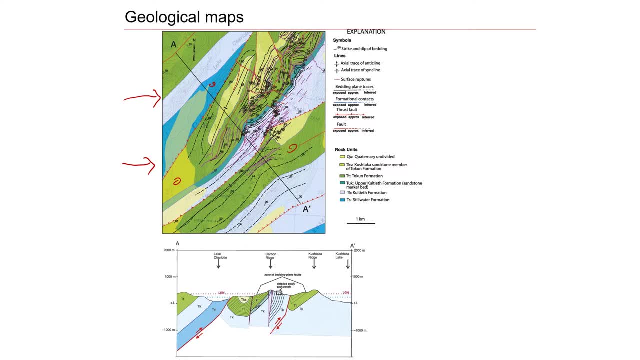 yellow color and green color. so the color shows the age and how much is left, And it also shows you the type of soil and rocks. Of course, when we first look at this map, we don't know what rocks or soils are there. 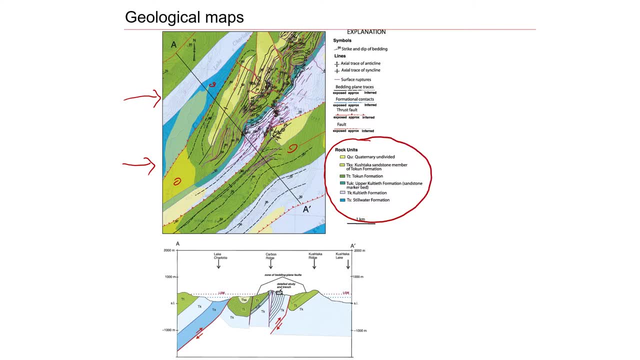 That's why we need to look at the legend. This legend explains all the colors and gives us the age of each rock or soil formation. Another important thing of this geological map is cross-section. Geological map only shows rock or soil units which are right on the surface. 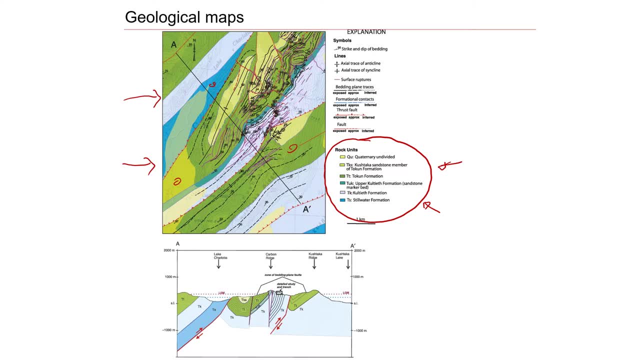 But when we will try to dig something deeper, we would like to know what types of rocks or soils are there. That's why we need to look at cross-section. So each geological map should come with a cross-section, And in this case it's line A in dash. 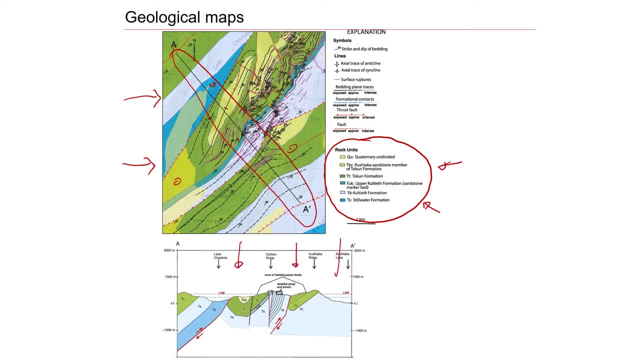 And the cross-section along this line is below. You can see that it shows different units here At different depths, And it also shows how they're placed in the space. This red line shows geological folds, which also flag areas where rocks or soil is weak and loose. 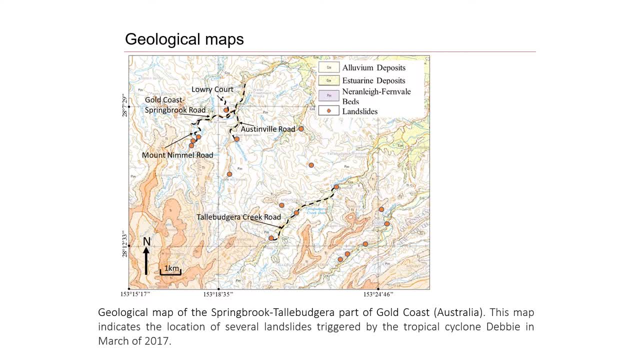 This is just example of our geotechnical investigation that we conducted a few years ago on Gold Coast. This is a map of Springbrook area And in this map you will see types of rocks and soils. And another thing that you can see on this map: 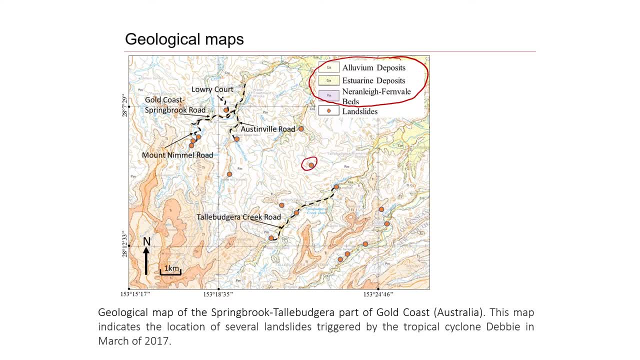 is the location of landslides. So you see all these red dots. This is where landslides occurred. So this is a very useful map because it tells us in what soil or rock formations landslides occurred, so that we can use this information. 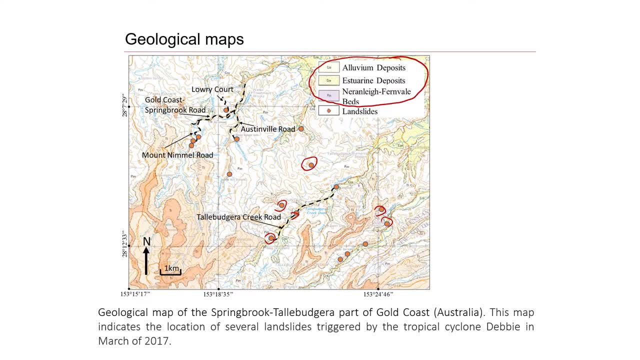 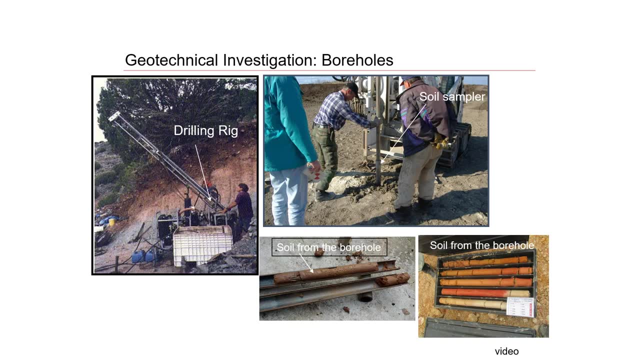 to predict the future landslides and try to mitigate them. To obtain as much information as possible, we would like to take some samples from underground. To do that, we will use boreholes. We need to drill many boreholes, as many as we are allowed. 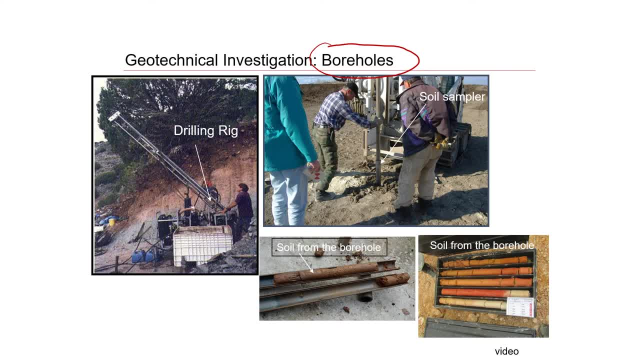 The only problem with boreholes is that they are very costly and we need to think twice where we need to place them. Unfortunately, sometimes we don't have lots of funds to drill many, many boreholes so that we can get a very good understanding of geological conditions of the area. 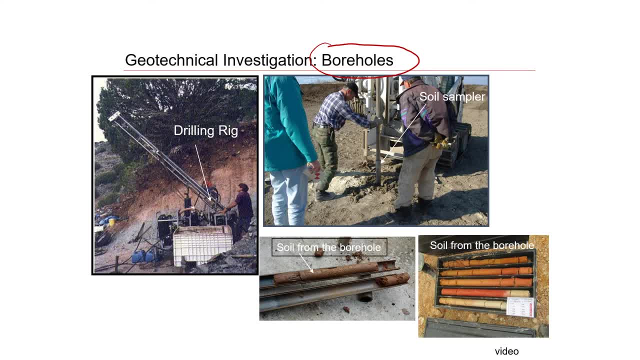 So we will drill as much as we can and we will collect samples. This is just an example of a sample that we collect from borehole. This is another example where we take many, many samples of soil and rock And after that we will examine that. 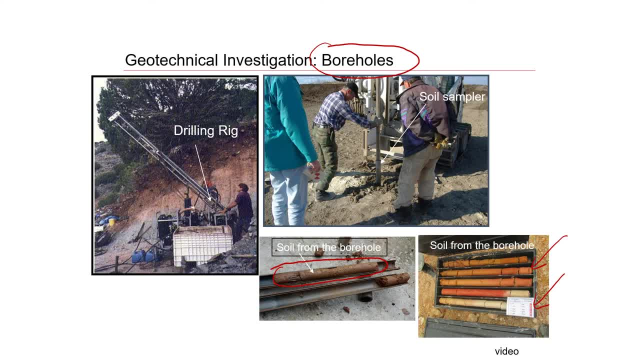 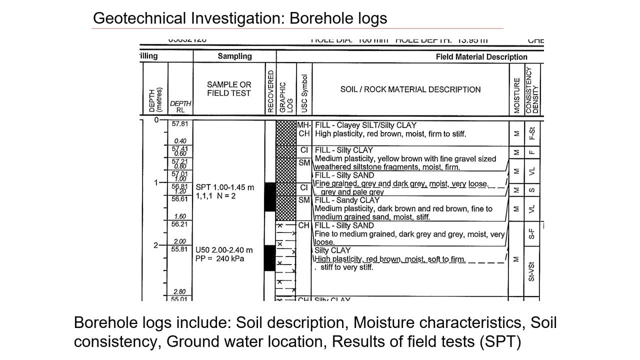 We need to see if there are any cracks, if it's moist or not moist. All this information goes to borehole logs. This is something that you would learn how to analyze in this course, And this is just a sample of a borehole log. 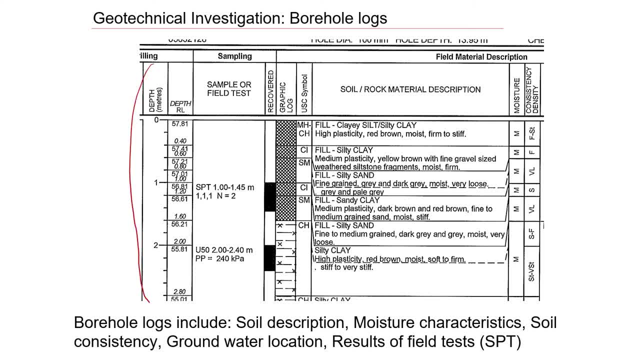 You will see that here on the left-hand side, the depth of drilling, so where we collect samples. Another important part of this borehole log is the depth. It is very important description. so description shows here so what we have. either it's a clay sealed, in this case, 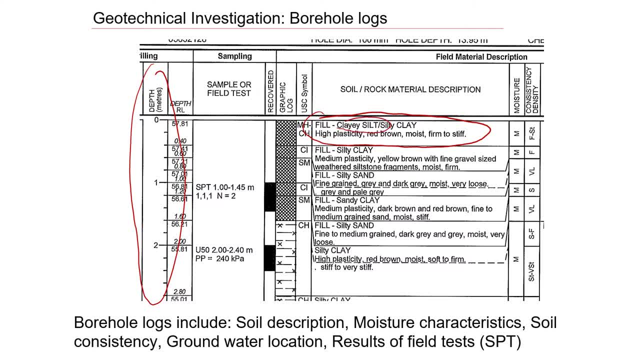 we have clay sealed and silty clay, then below we have silty clay again, and so, on another important part that we would like to know from this borehole log, it's the amount of moisture in soil, which is shown here, as you will find out later, if soil has lots. 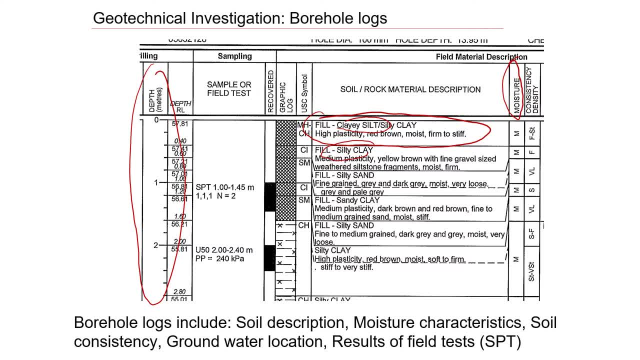 of water in it, it will become moist and this is not very good property of soil. so in this case you will see that at the top soil is moist. then also, if we go down, all the soil is moist. most soil is typically weaker than any dry soil. 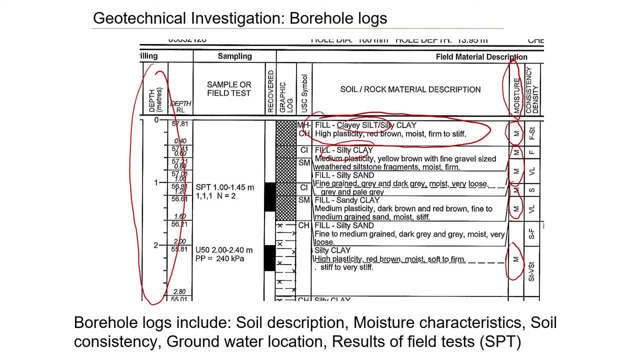 of them. so another important thing is consistency, or density. it will show the consistency of the soil in the field. it can be firm, it can be loose, and there are different symbols that are given in the legend for each borehole, so just remember that borehole logs. 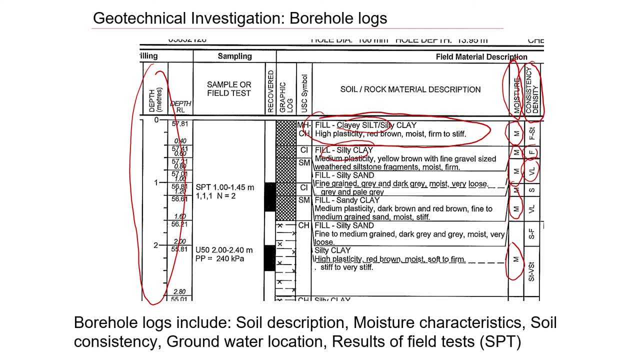 will give you very important information that you will need to know to draw a geological cross section. another thing that i didn't mention is results of spt test. spt test will give you some idea about the strength of soil at certain depths. so in this case the depth is one meter, then around two meters. there was another test. 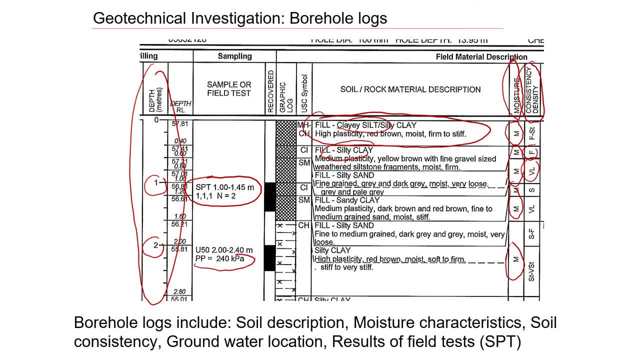 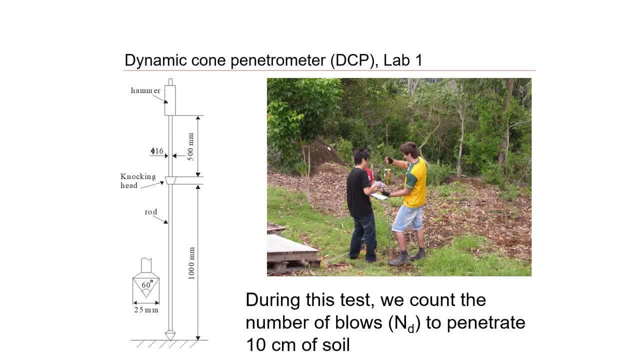 excuse me. so there was a test here. so there was pocket penetrometer test here, not SPT. If we cannot drill boreholes because it's very expensive, we can do another test, which is called dynamic on penetrometer test, and this is something that you would learn how to do in the first long meter. The test is pretty. 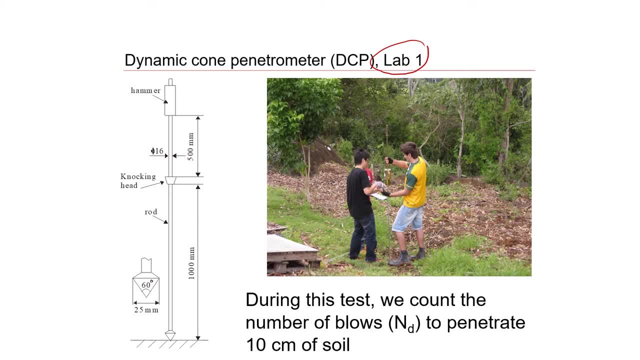 simple. we can bring this equipment, which is called DCP, to any parts where we would like to investigate. it can be slope or it can be area where we cannot bring borehole drill. So the test is shown here in the picture. so this is DCP. we put it. 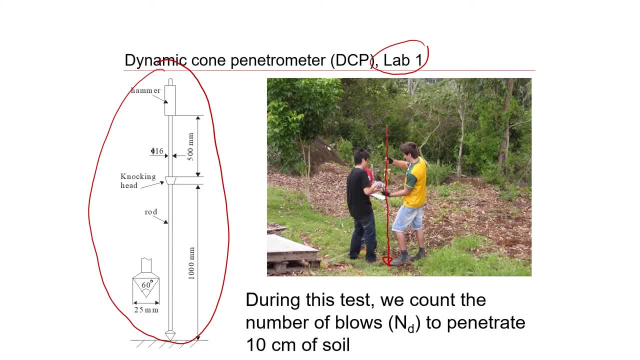 on the surface and then we use hammer, this hammer to drive this DCP inside the soil and we just measured the resistance of soil to the penetration of this cone and we upload this results. this is something, again, that what you would learn how to do in the first. 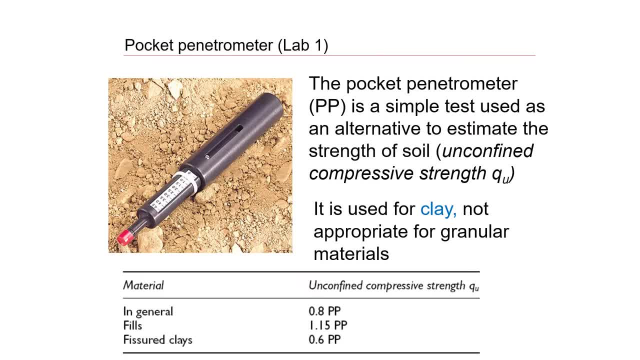 laboratory Pocket Benefonder, as it's another very useful tests. it may not be very well known why this, for this very purpose- this Milwaukee next to wound- very reliable. that's why we would like to do at least three measurements of each soil. the test is pretty simple. this is pocket penetrometer. we will press this part of the 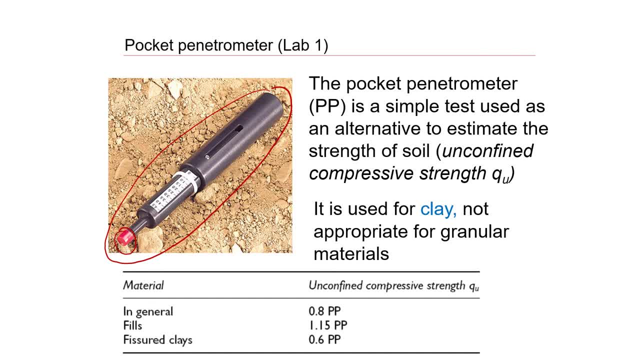 pocket penetrometer against the soil and we just measure source resistance using the scale. here, as i mentioned before, we will need to do three tests and we will get an average value. the good thing about this pocket penetrometer test is that it correlates with the unconfined. 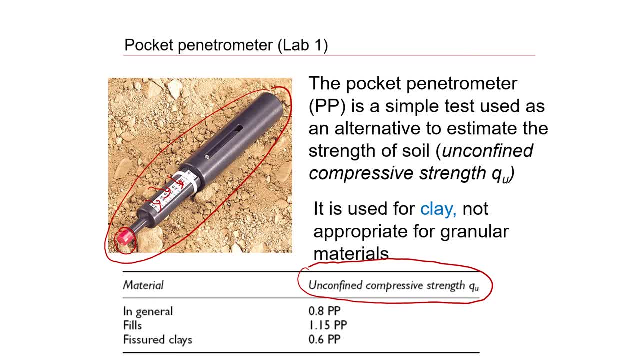 compressive strength of soil and these are the correlations for each type of soil. typically, when we work on the site, we deal with general soil, so in this case this is going to be the relationship. so it's 0.8 times the value of pocket penetrometer test when we work with fields. 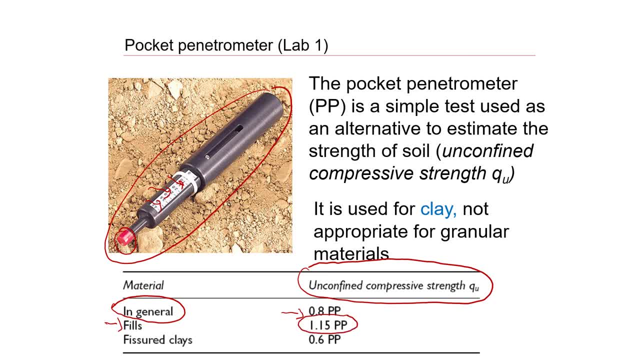 the relationship will be slightly different, so the coefficient will increase to 1.15. this soil is mostly done for soft material such as clay. unfortunately, you cannot use it for sand. it just doesn't work. also, we don't use it for rock samples. for rock samples we have a similar type of equipment which is called schmidt. 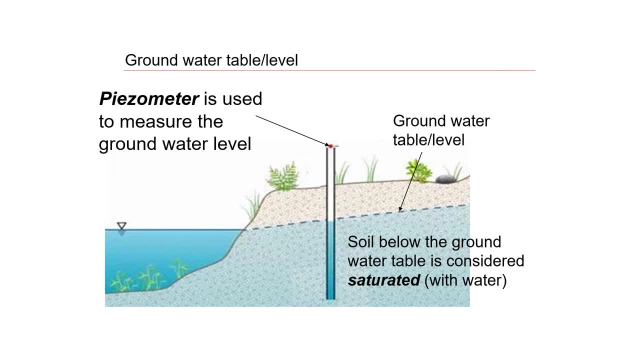 or an tip might help us deciding which soil we are: Kakashi, mmo Lily or amor Smith, which are ontanite, and which ones are as wanted as wezoides or dropping from the soil. at one point we can adjust this super volume with the провер, the ratio. I will go down a bit further and if it works we give a. 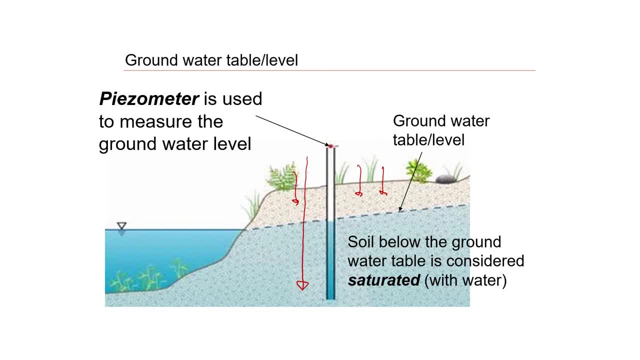 blow at that point and press thejiang coming down, and возможно we'll do it. even on flat soil see that the soil is filled with water. so we would like to know the level of that water, and this is what we call groundwater level. we use this symbol to define this groundwater level. 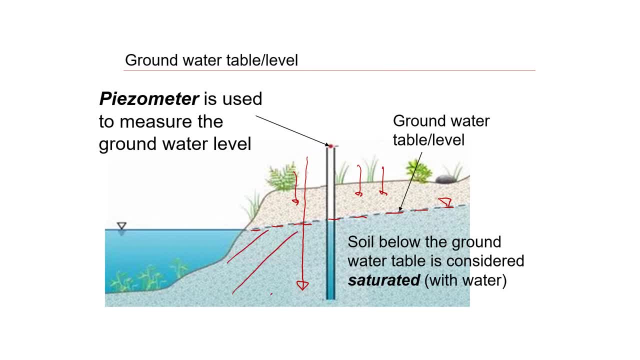 so what we assume is that the soil below this groundwater level is saturated, so there is water in the soil. here, on the top above the groundwater level, there may be some water in it, so the soil can be moist here, but there is no groundwater level. you will see. 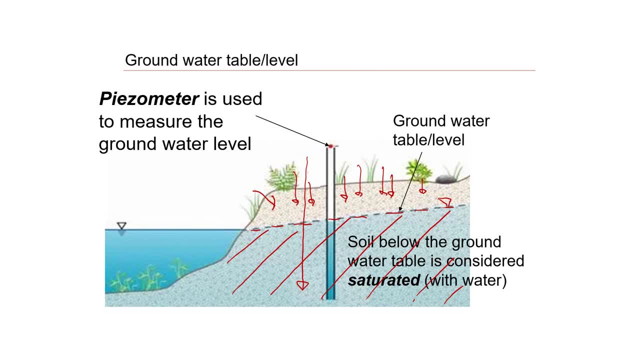 later. that groundwater level will have a strong effect on the stresses in the soil and this is why we need to know where the level is. to do that, we will use a piezometer, so we will drill a borehole or drill a hole here and we will install piezometer.